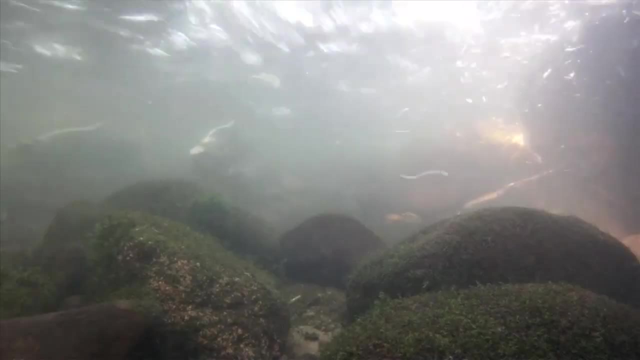 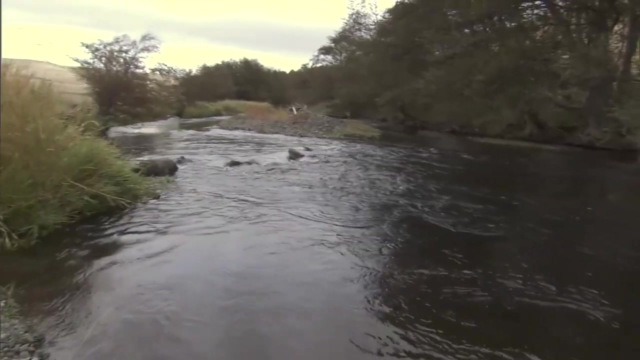 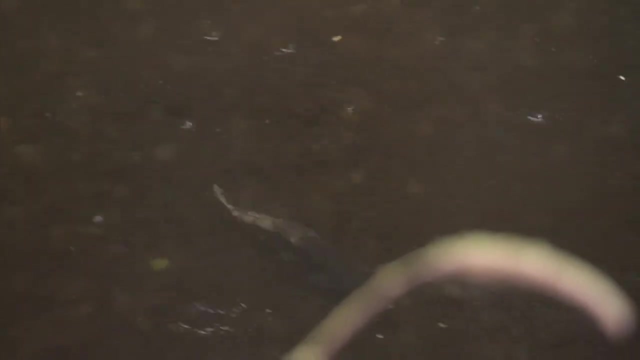 back to their birth stream to reproduce. Some fish travel hundreds of miles upstream before they reach their spawning grounds. At their birth stream, male and female salmon pair up to breed. The time of breeding depends on the location and the population of the salmon. 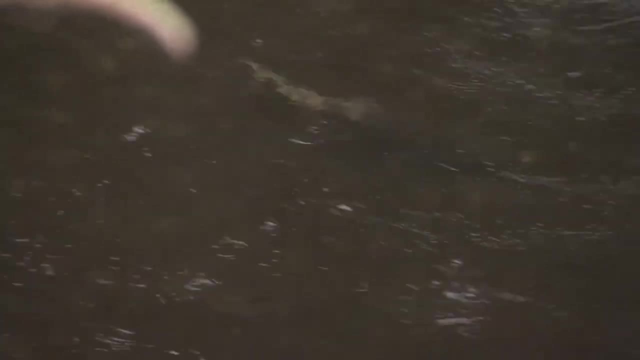 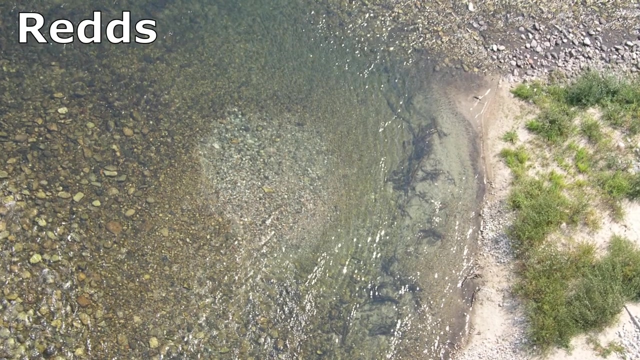 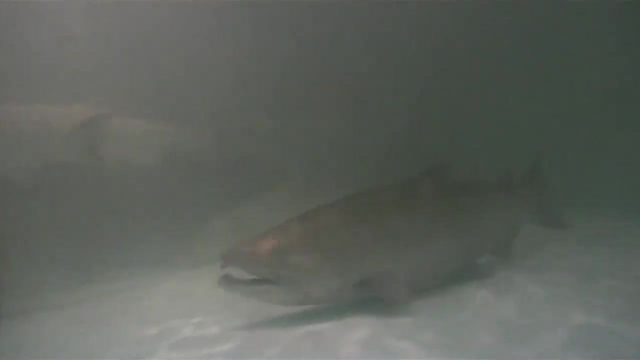 But most breed in the summer and fall. The returning chinook salmon dig out gravel nests, called reds, on stream or river bottoms where they lay their eggs. A female will deposit thousands of eggs before the male releases his sperm. A female chinook salmon can deposit. 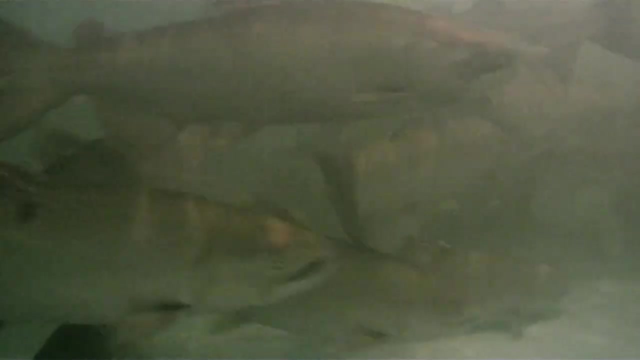 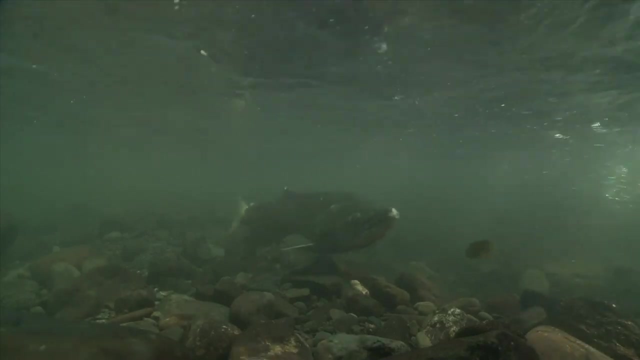 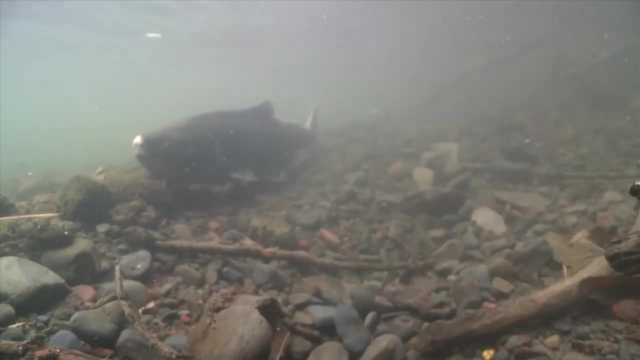 anywhere from 3,000 to 14,000 eggs in a nest. The reds can be up to 10 feet in diameter. After mating, the male and female guard the eggs in order to protect them from predators. Chinook salmon do not feed during their freshwater spawning migration. 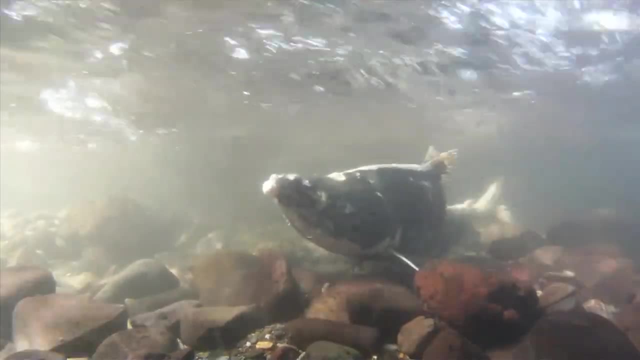 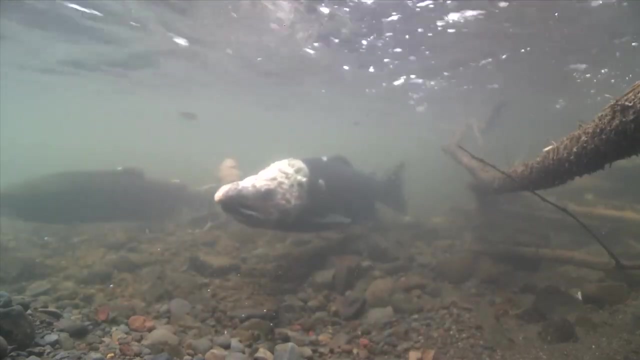 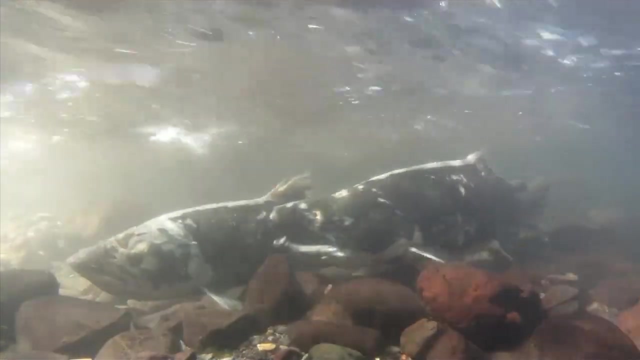 They burn a lot of energy migrating, breeding and protecting their eggs. All chinook salmon die shortly after spawning, before their eggs even hatch. The eggs hatch in spring Because they die after spawning. their carcasses provide abundant food and nutrients to plants and animals, including tiny aquatic insects and other invertebrates. 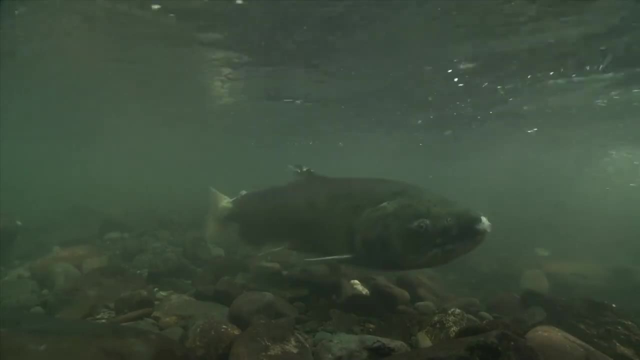 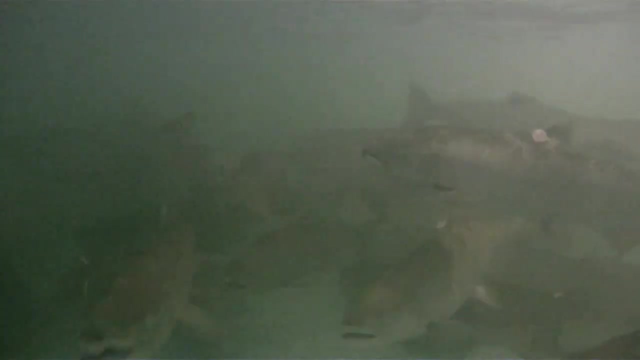 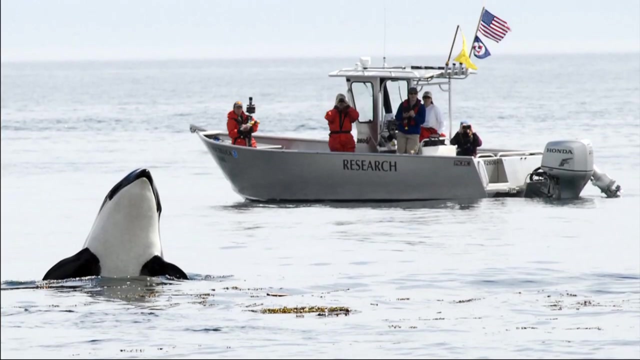 that in turn provide food for other animals. Chinook salmon are a vital food source for a diversity of wildlife such as killer whales, bears, seals and large birds of prey. They are the primary food source of the endangered southern resident killer whales During their life cycle. salmon transfer energy to the environment. They are also a source of energy for the environment. They are also a source of energy and nutrients between the Pacific Ocean and freshwater habitats. In areas that have experienced dramatic declines in salmon, there is a measurable deficit of nutrients to help support the ecosystem. 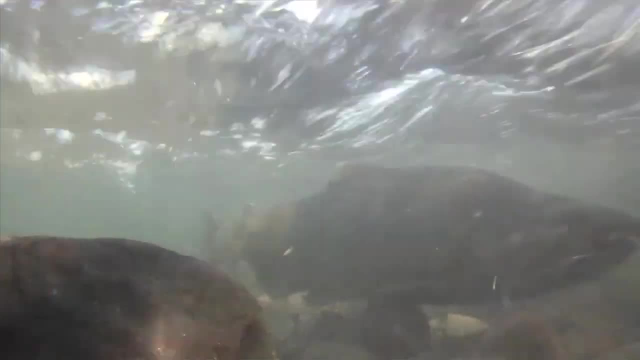 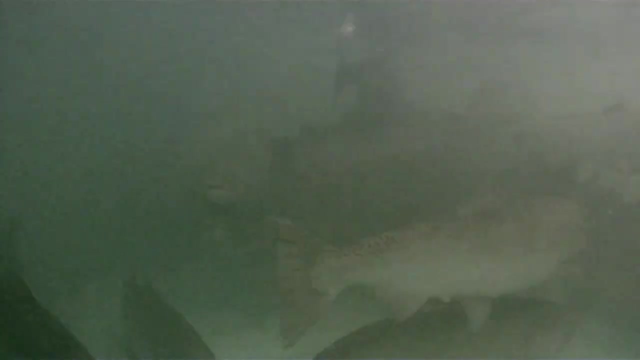 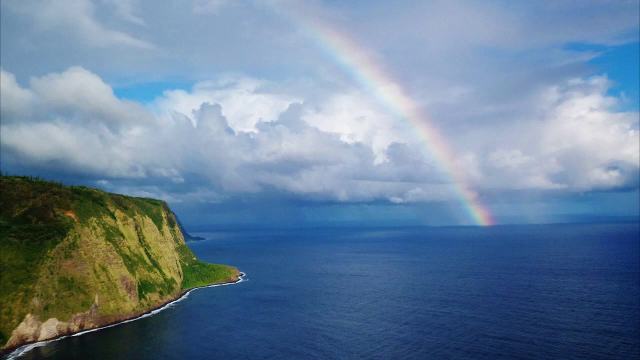 The salmon are commonly harvested commercially and for personal use. Some of the threats to chinook salmon include blocked access to spawning grounds and habitat degradation caused by dams and culverts, along with overfishing of their populations. For more marine facts, click the SUBSCRIBE button.